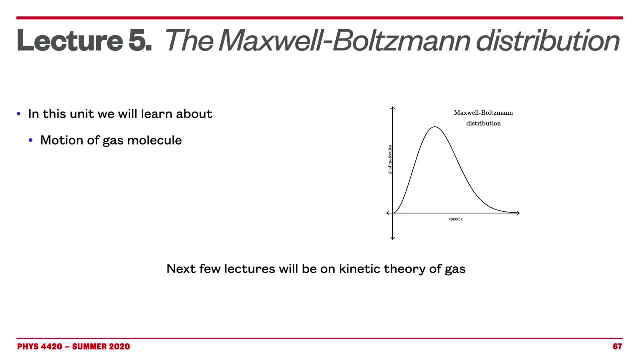 Welcome back. Now we move to lecture five, And this is the first lecture on a series of lecture where we'll be talking about the kinetic theory of gas. So kinetic theory of gas is essentially understanding the distribution of velocity, understanding how those properties relate to thermodynamics, thermodynamics and thermodynamic properties. 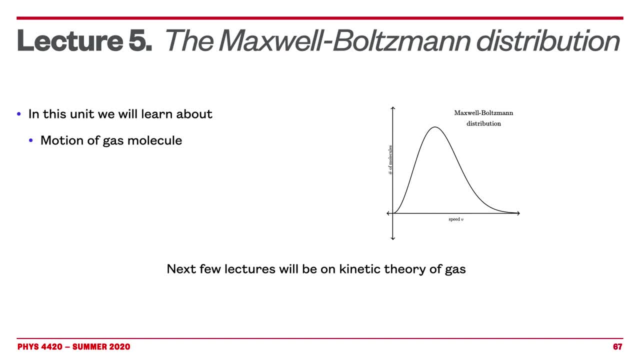 And the big thing we are going to do in this lecture- in fact, the only thing we are going to do in this lecture- is to derive the mathematical expression for the Maxwell-Boltzmann distribution And, spoiler alert, the figure there that's on this slide is the result that we are going to obtain. 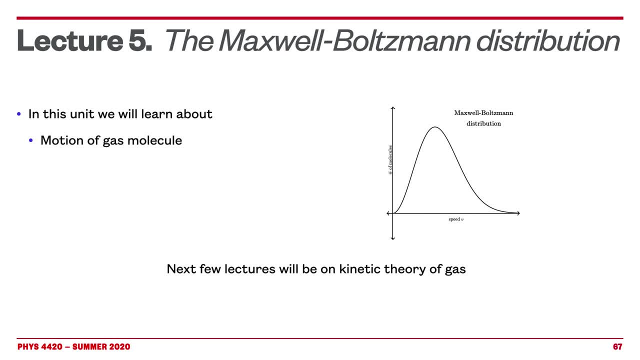 This is a very important notion And again I'd like to show you how we build in this course, The distribution. of course, by now You should be familiar with the fact that when I talk about distribution, I'm really talking about probability. 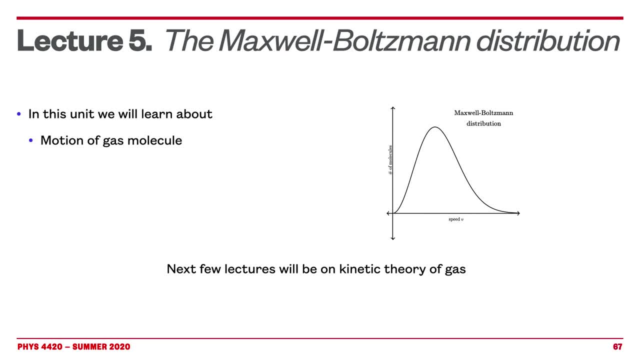 So that's going to give us the probability of finding the gas molecule at a certain speed, in this case right. And so on the y-axis you will have the probability, or in other words the number of molecules really, and on the x-axis you have the velocity. So the distribution here, which is a distribution, 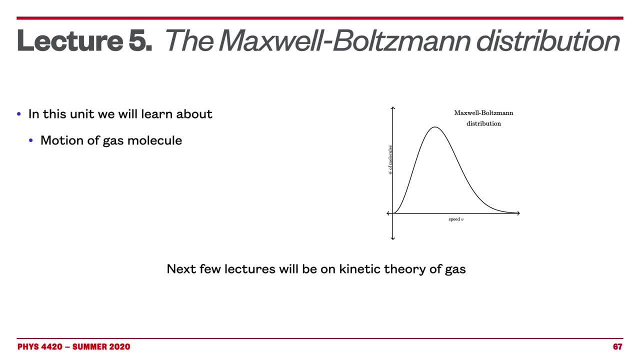 that's going to depend on on the temperature, is going to tell us essentially at what speed we should, with what probability we can find gas molecule with a given speed And we will find that those properties are going to be relatable to thermodynamic properties. We are going to do that, but we are going to prove this first: how we can calculate this Maxwell-Boltzmann distribution. 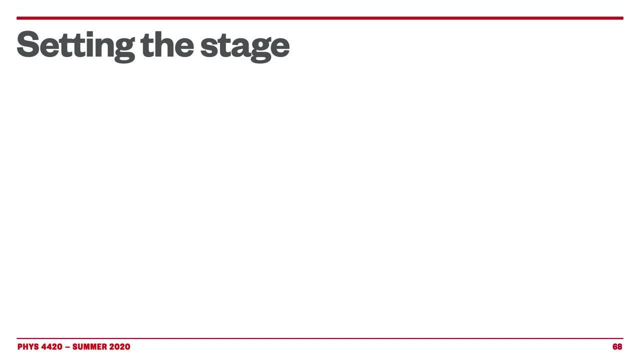 So let's first set the stage Again. we are going to work with pretty much ideal gas. we suppose that they are monoatomic. The reason why we do this is because we don't want to have the complication due to the to the rotation of the gas on itself or it's vibrational, For example, if you have a diatomic gas, there is a vibration. 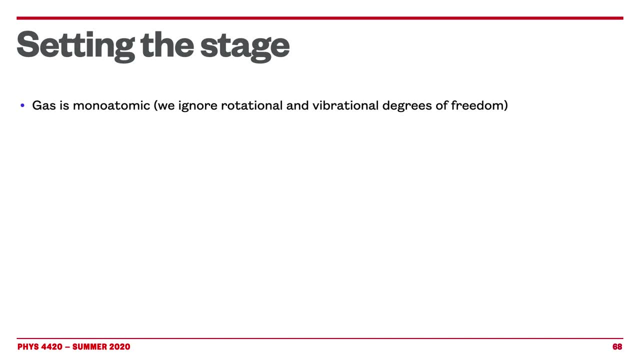 so there's some energy that can be stored there. We're not going to do that. We are just going to suppose that the only energy that's going to be in a gas molecule will be due to its kinetic energy. That's basically the idea. So we are making things a little bit simpler and it will add degrees of freedom. 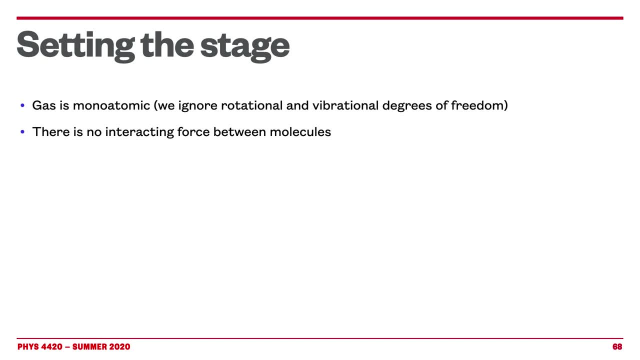 later, as we move along in this course, There is no interaction. So, as I said, there is no interaction between molecules, just the same as we saw for the ideal gas. That means that the only energy, as I just mentioned, is the kinetic energy. 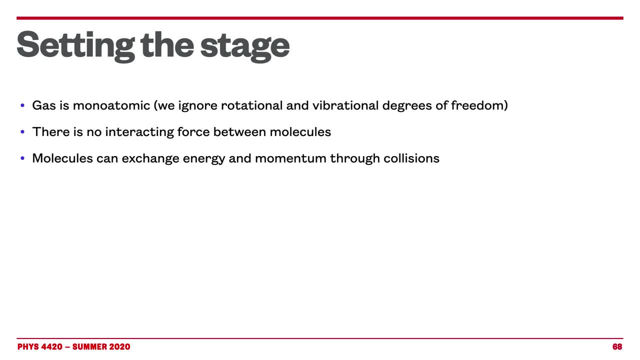 They can exchange energy, though. The molecules can exchange energy through collisions. So, as you know, when you have a collision you exchange energy and momentum and the conservation of both during the collision. as you know from elementary physics, We will only consider linear motion. of course, In this case, again, we will use the Cartesian coordinates. 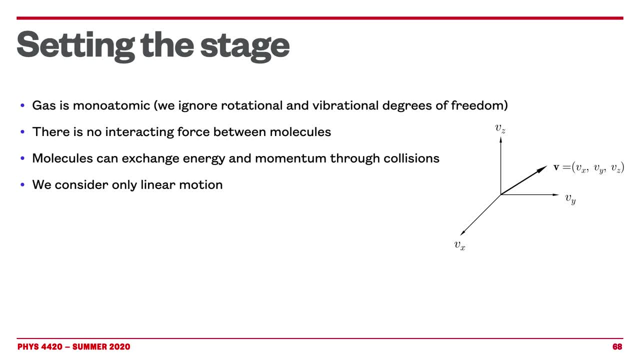 where in the velocity space vx, vy and vz are orthogonal and we do find that the vector- velocity vector- will have components vx, vy and vz And of course in that case the energy, the kinetic energy, is simply the sum of 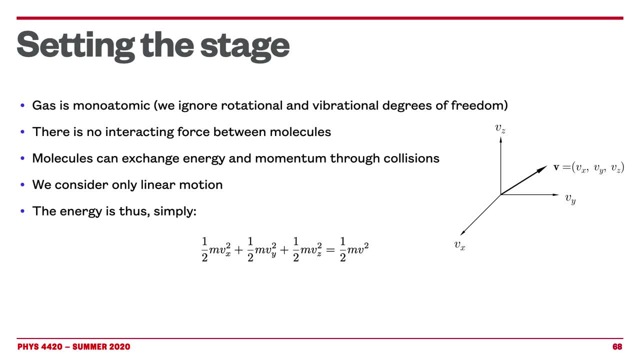 mv x square plus half half mvx squared, half mvy squared and half mvz squared, For a total of one half mv squared, where v is the length of the vector in Cartesian space. something fairly elementary. So what we just to set the goal of this lecture. 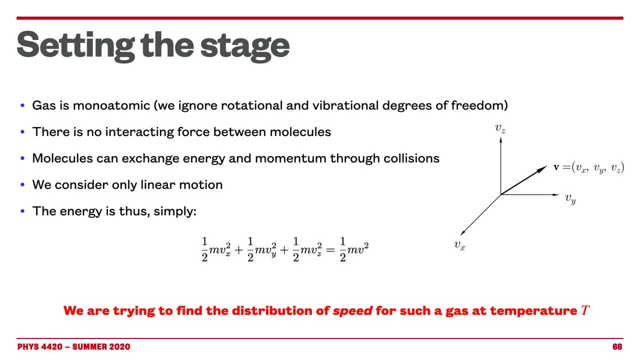 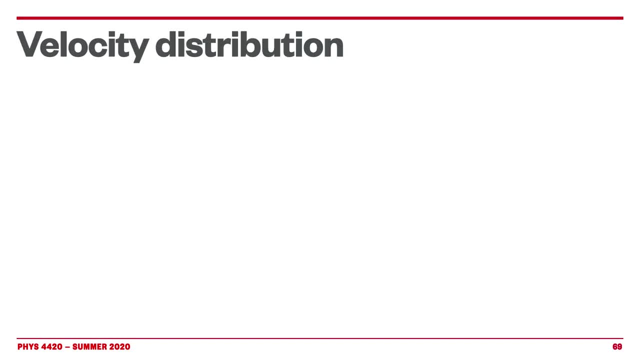 is to try to understand the distribution of speed for such a gas at temperature T. So we are going to look at that. So let's have a look at the velocity distribution. And this is essentially the most important slide of all, because it's going to translate what we've learned so far into this particular problem. 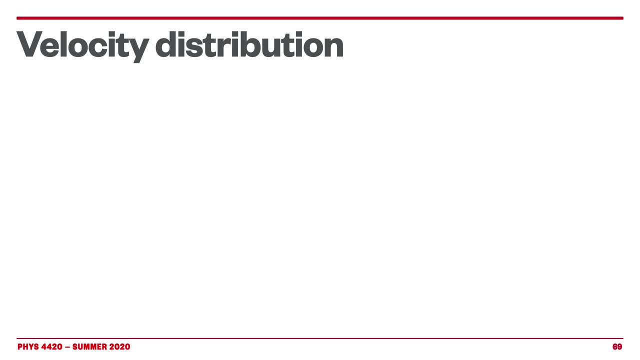 So imagine that you have a gas or molecule and we are going to work in a canonical ensemble with constant temperature, And so we imagine we are going to imagine a single molecule inside of the gas. So we are going to imagine a single molecule inside of the gas. 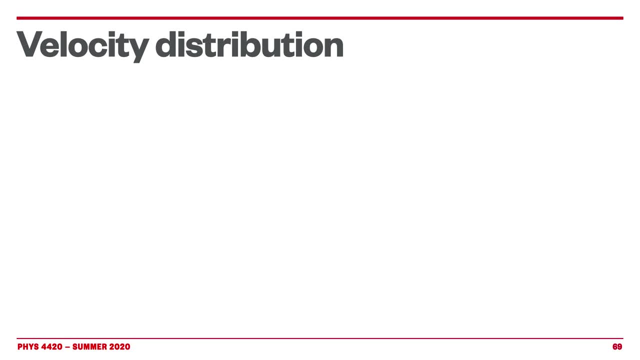 So, basically, there are many, many molecules in the gas, but we are going to look at the perspective of a single molecule And for that single molecule it looks like the molecule is in equilibrium- in thermal equilibrium with all the other, with the rest of the gas. 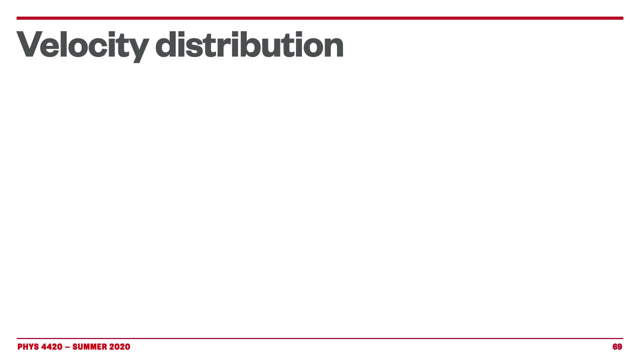 which we're supposed to have many, many, many molecules. So that looks like the definition of a reservoir is pretty good is certainly obeyed. So that means that if we can do that, we can use the Boltzmann distribution. the Boltzmann distribution is going to give me the probability of finding the molecule in a certain energy state. 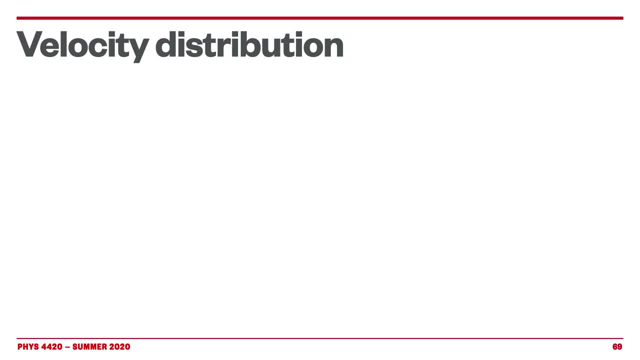 But energy states here are defined by the kinetic energy. Remember, the Boltzmann factor is simply a factor that corresponds to the energy of a particle divided by kT. So basically that's what we will be doing here. We'll consider each molecule embedded in a system connected to a bath. 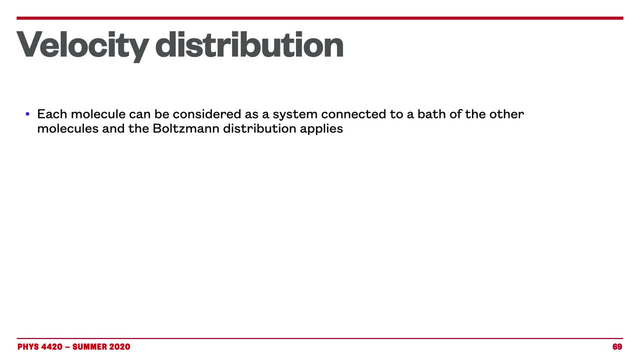 and the bath will be all the other molecules. So remember the bath, the heat bath and reservoirs. Reservoirs are the same thing as synonymous, So of course the Boltzmann distribution applies. And remember, this is a distribution, this is a probability. 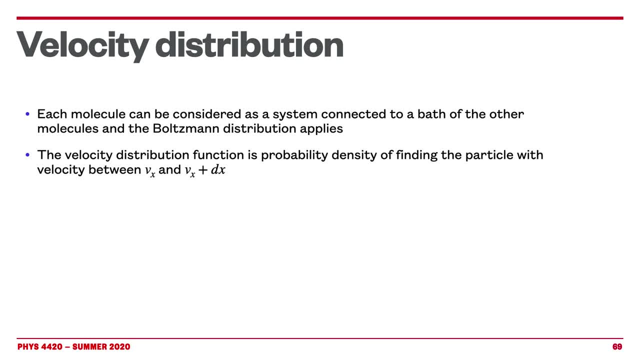 but because we have a continuous function, a continuous variable, which is the velocity, we have to look at the probability density. So, in other words, we get the probability not of finding Vx, but the probability of finding Vx, and Vx plus dx. 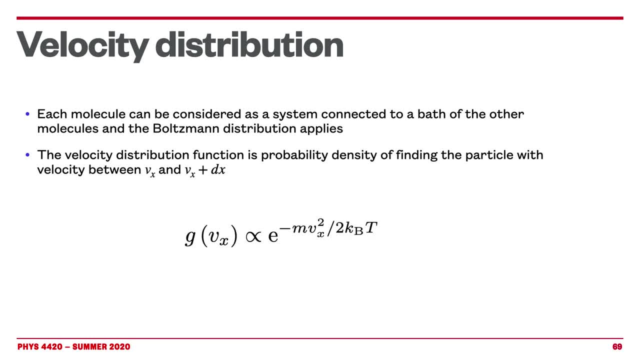 And that probability is going to be proportional to, to a Boltzmann factor that I've just wrote there, where the energy is the kinetic energy. So you have mVx squared divided by 2.. Okay, That's the most important thing, because of course we know what this looks like. 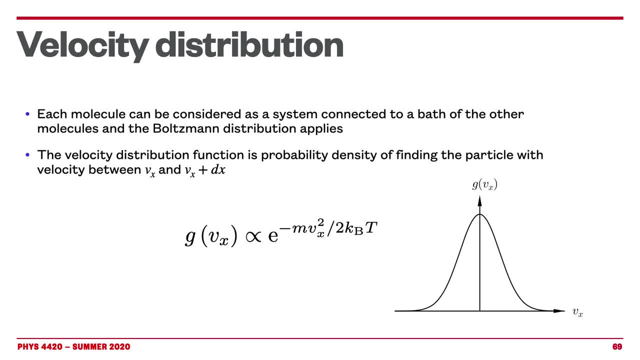 This looks like a Gaussian right. If you plot the distribution as a function of Vx, this is a Gaussian, Which is good news, because we know a lot of formula for Gaussian integration and that means that we will know a lot of things analytically. 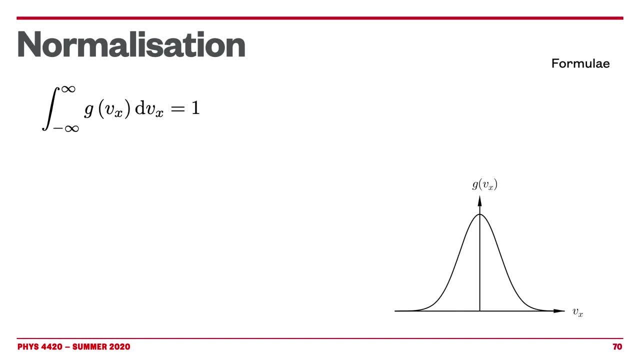 In particular, we can normalize this function, which simply means that the total sum of all the integral of the integral- I mean the total, the integral over all the possibilities, will give one. So, in other words, we know that all the particles will be. 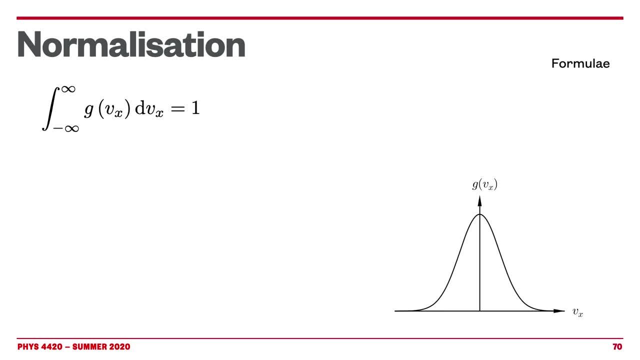 will have velocity, basically right, Or including zero. Okay, very good. So we are looking at this as only one dimension There. the button there on formula would lead me to the formula on the integral using Gaussian. I'm not going to go there because we've done it before. 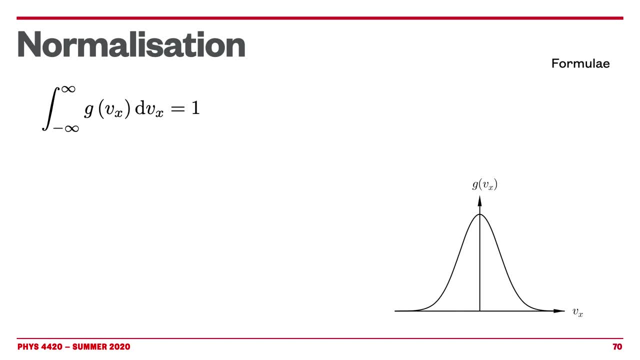 but this is for those who are following with the book. This is in the appendix or you can find any table that have the integral for Gaussian. We're not going to spend time on this. It's fairly elementary. The point is that that integral is going to give me a number. 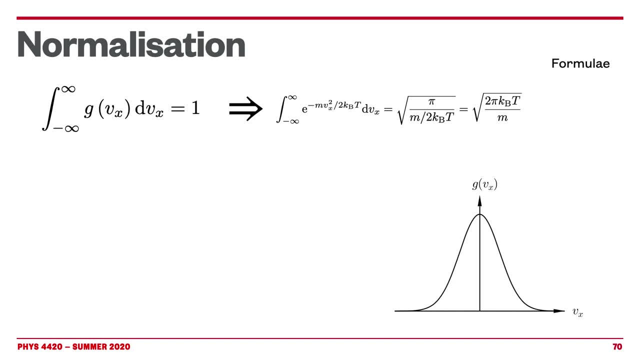 So the integral of what I found in the previous slide gives me a number which, since it's not one that, means that my system, my distribution, is not normalized. So all I have to do is to divide by that this integral, and I end up with. 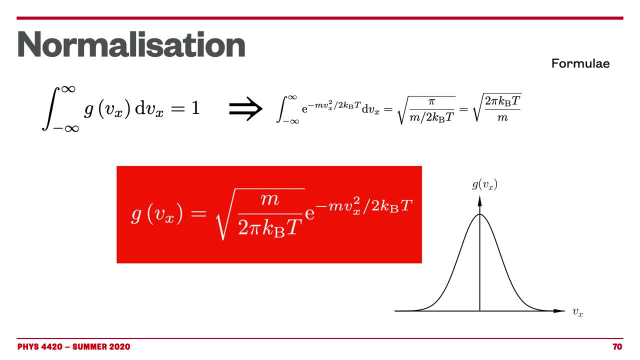 this equation, which is a very important equation, Of course, it's going to give me the probability density of finding a particle. So GVX times DVX would give me the probability, then the probability of finding a prop particle, So a gas molecule of gas. monoatomic molecule of gas. 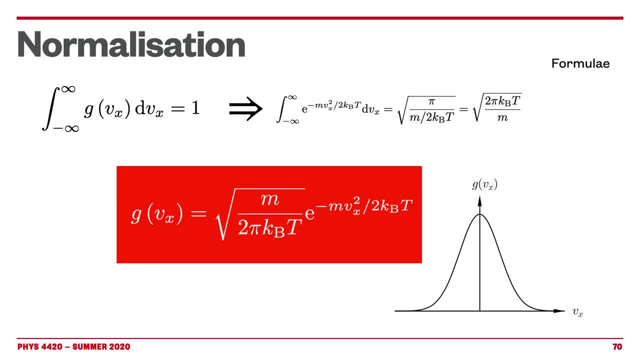 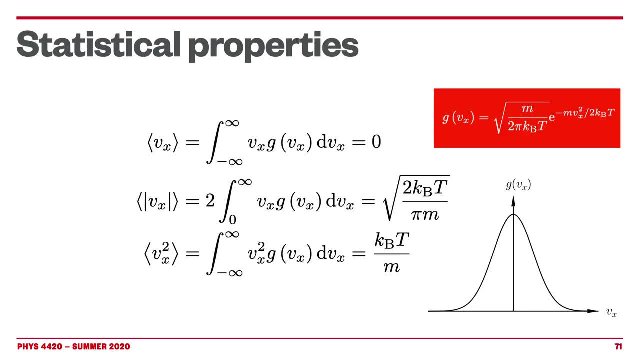 between VX and VX plus DX. So this is this: is this come directly from the Boltzmann distribution? Again, each time we have a distribution probability distribution, we can calculate the number of statistical properties or the typical ones. That's a good exercise, again to apply the rules. 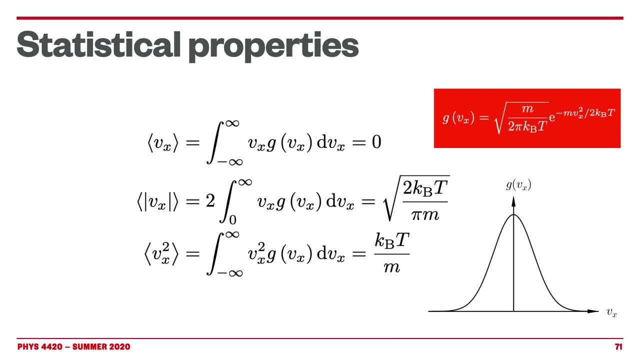 the mathematical equation for Gaussian integrals can calculate the expectation value. Of course we have a Gaussian, So we know the expectation value is going to be zero, right As always, because of the symmetry around: VX equals zero. What's more interesting is to calculate the expectation value of the absolute. 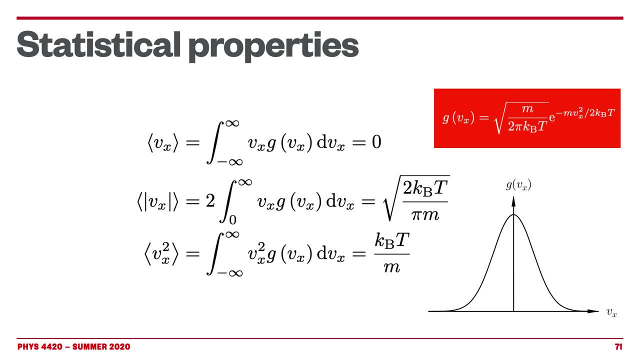 value of Vx And, of course, also the expectation value of VX square. We know that the expectation value of VX square is going to be important for our purpose because we know that the kinetic energy is MVX square over two. That means that it looks like it's important if we want to know the expectation. 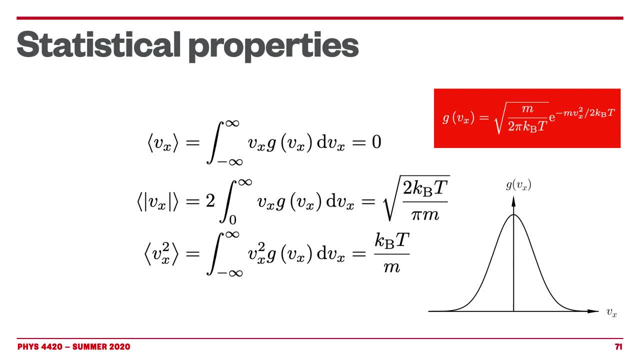 value of the expected power of X of the energy. it looks like it's a good idea. and, of course, again, another spoiler is that we find already that the expectation value of vx square is kbt over m, so that's already telling us about what would be the expectation value for the kinetic energy along the x-axis. of course it. 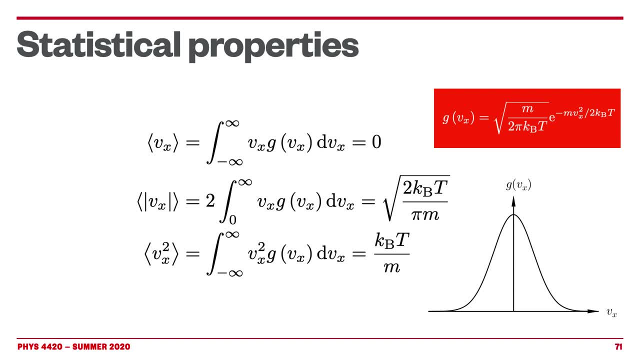 would be kbt over 2, since, since the kinetic energy is mvx, square over 2. anyways, i'm jumping the guns a little bit here, so we'll get back to that in a few minutes. okay, so this is just in one dimension. so this is the probability. gx times dvx is the probability of finding the gas molecule. 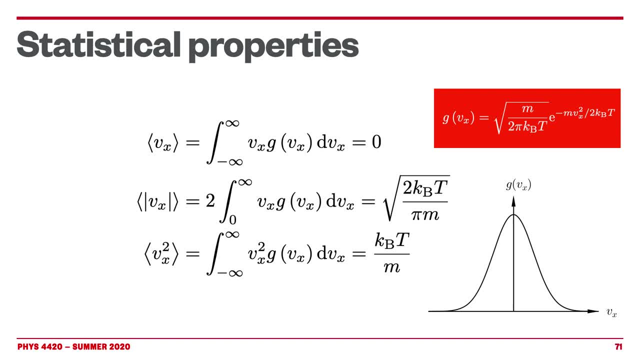 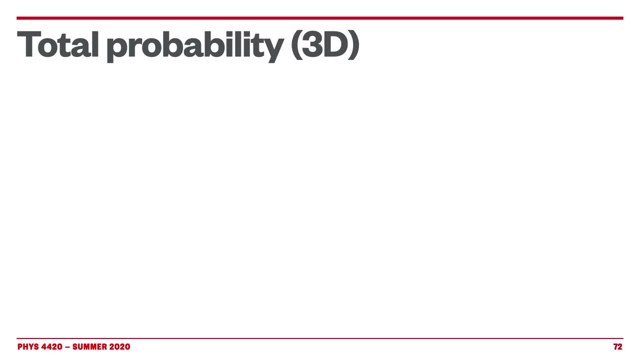 between velocity vx and vx plus dx. okay, that's not quite what i want to do, because we live in a three-dimensional world, at least in cartesian coordinates. so what i'm interested in is a total probability, and here it's a math fool, but i'm going to say it anyways. that's the probability. 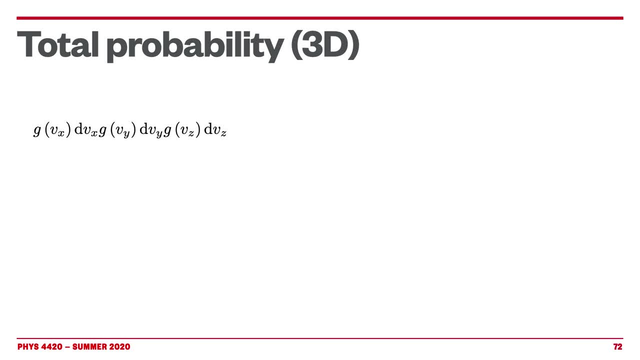 that the particle has a velocity along x, that's between x and x plus dvx, between vx and vx plus dvx times the probability of finding that particle with the velocity along y, between vy and vy plus dvy times the probability of finding that particle velocity along z in. 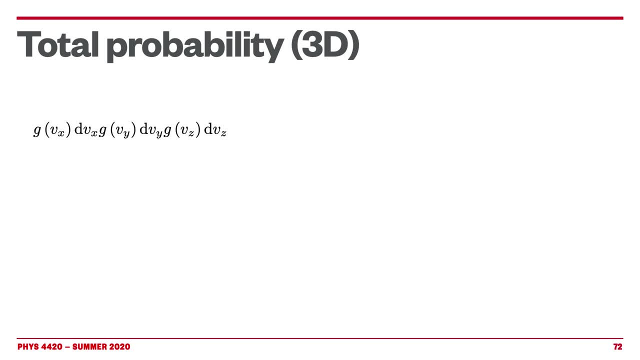 vz and vz plus dvz, that's it. so it's a product, of course, because probability of compounded uh processes is always given by the, by the product i. the good news is that in my treatment that i did in the previous slide, i just picked an axis randomly, but it could have. 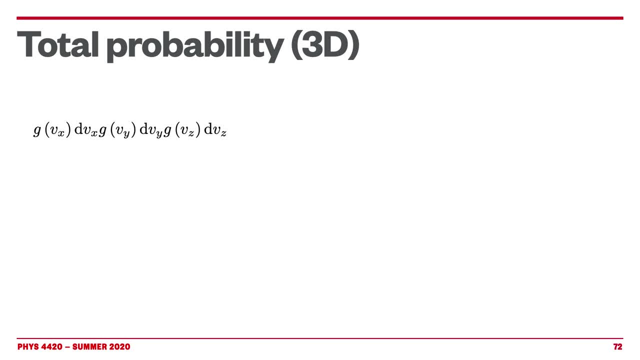 been any other axis. so the math is described the same way. in other words, we get, we can replace the gvx and gvy and gvz, but what was found in the previous slide? what's nice about this, of course, is that, because of the exponential we can, of the product of the exponential is the exponential. 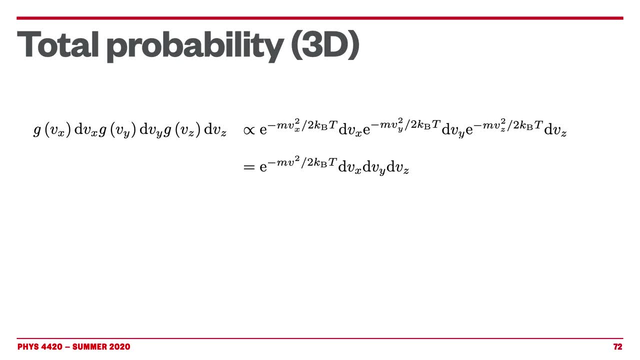 of the of the sum, and i end up with, uh this formula, which is: which is nice, uh. so the probability uh of finding uh the particle in that box in in in velocity space, right, remember, it's a box that's between vx and vx plus dvx, vys and vy plus dvy, vz and vz plus dvz, so the probability of finding it, 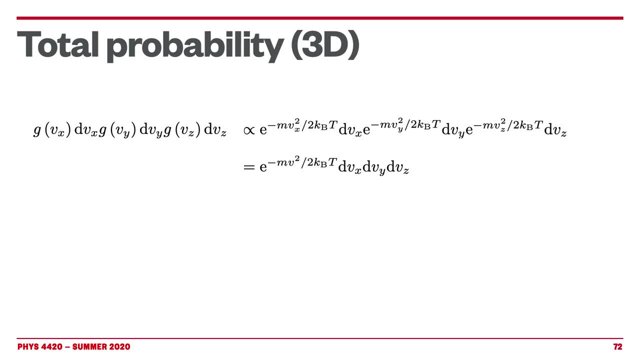 in that box is given by this formula, where v square is vx square plus vy square plus vz square. so that's all very nice. the problem is that that probability is essentially useless, because this is the probability of finding the particle in a small box. but what i'm really interested in is the probability of finding the 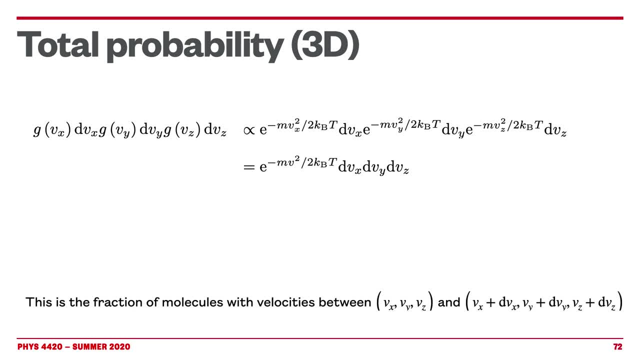 particle with a given velocity or actually given speed. right, the scalar version. so what's the probability of finding the particle with a certain speed, like, say, five, seven, okay, something like that. so so that's that's not quite what i have here, because this one is just the probability of 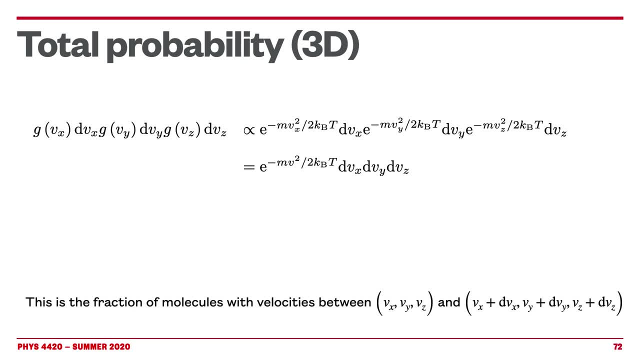 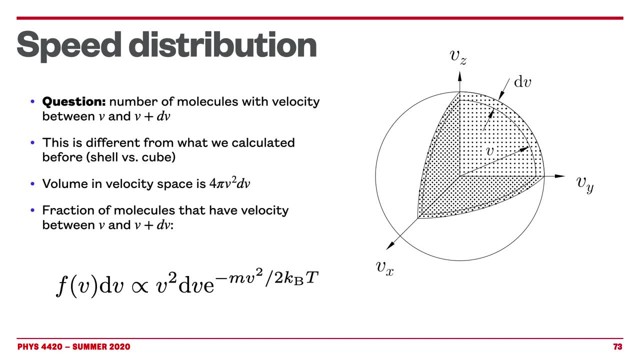 finding a particle in certain cube in the in the velocity space. so instead what i need to do is: in that velocity space is i look. i have to look at all the places where the velocity vector end up is in a shell of radius v and uh, thickness dv. 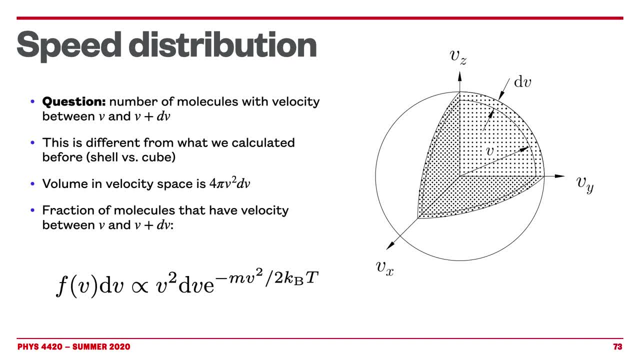 right, that would be. that would give me, if i can find all the particles in that shell, uh, external shell, then i would. i would, of course, get the probability of finding the particle between of with speed v, between speed between v and v plus dv, and of course this calculation is is not very complicated. 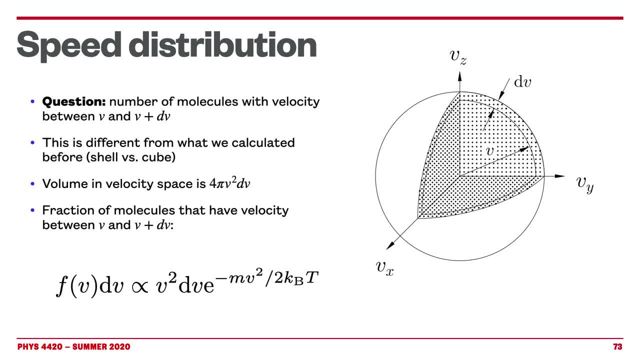 to do when we remember that the volume of that shell is going to be the surface of the shell times its thickness and, of course, the surface of of a shell it's. it's basically the surface of a of of the sphere, which is 4 pi v square, and the thickness of the shell is dv. so the volume of the 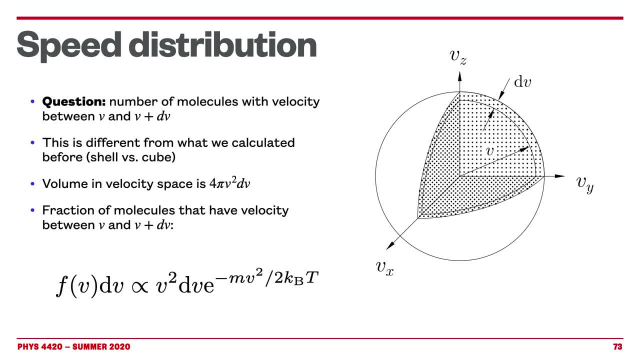 shell is 4 pi, v square, dv. and i know the probability, uh, the probability that i find, uh, to find a particle in in any of the box that that i just described in the previous slide on the shell is the same. it only depends on the speed, right, it only depends on on v square. so that allows me to. 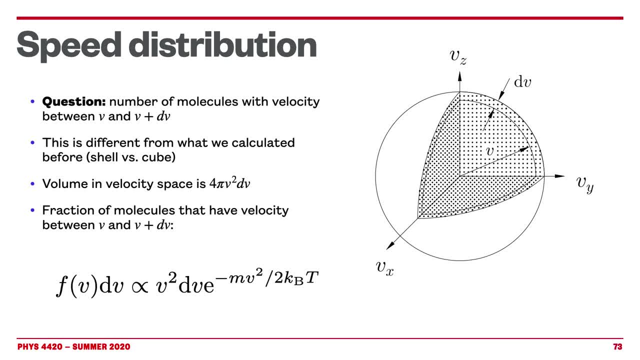 write, of course, the, the equation that's on the bottom left of this, of this uh, of of this slide, there is no 4 pi, because we have a, this is proportional right, we have the proportional sign, so we, we can leave the v, the 4 pi, within the proportional sign we will need to to uh, we are. 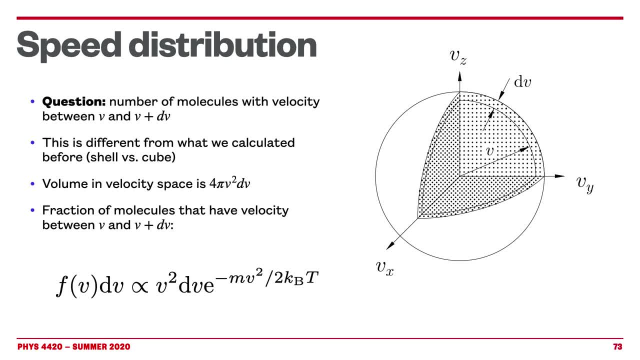 going to need to to normalize anyway, so let's not worry about that. what matters, though, is that now, the probability of finding the gas molecule between v and v plus dv is v square times the e minus mv square over 2 kbt, so that's the v square in front. there just comes from the fact that we are 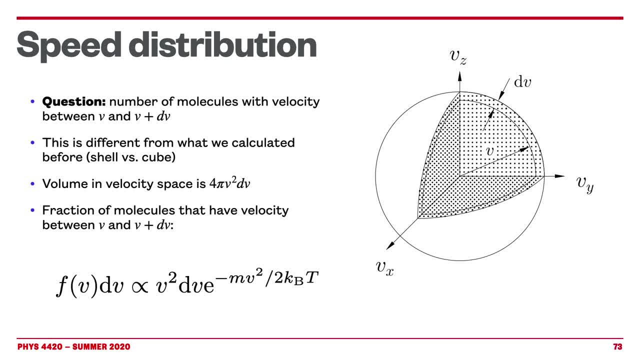 integrating over a sphere. all right, so that's very usual, that what we have, that each time we work in in over, uh, we are interested in distribution of, of length or speed, versus the distribution of the component. we always, we often end up with a quadratic term. that's simply coming from the 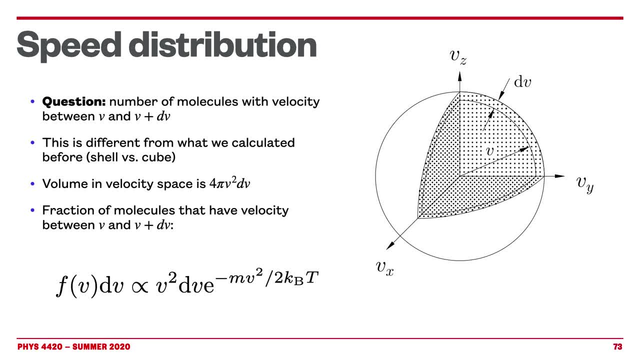 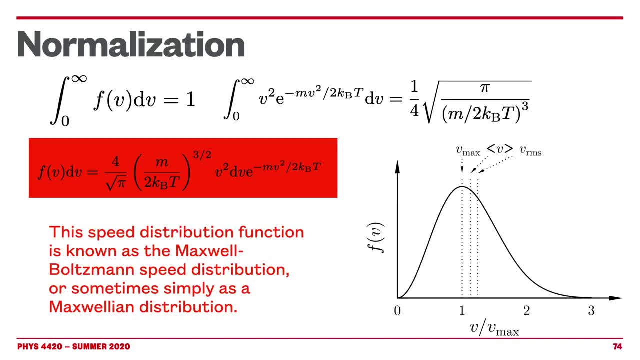 surface of the shell that we are integrating over. so that's nice, we have this and we're almost there. this is this, almost. this is almost the maxwell-boltzmann distribution. to get the maxwell-boltzmann distribution again, we want a distribution. therefore, we need to normalize. 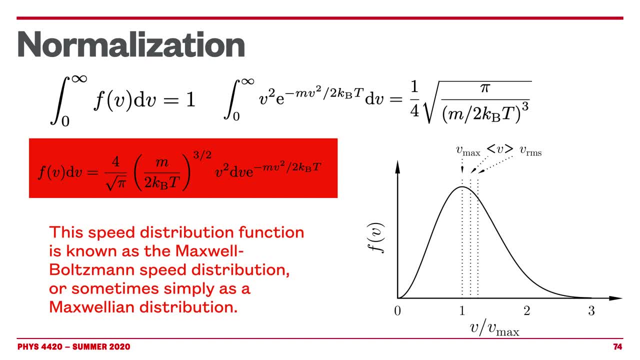 and to normalize, we integrate this one more time. this integral is actually fairly straightforward when you have the, the, the form uh, the formula from, from, from the table, from mathematical tables, and you end up with the, the pre-factor um, and the pre-factor is important because the pre-factor is. 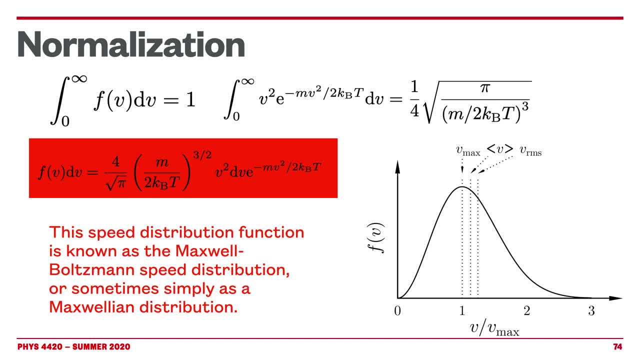 going to be to give you to make sure that it's a true distribution where the total probability is equal to one. okay, so what's nice about this? now- and this is the what's in the red box, because it's very important result- it's called the maxwell-boltzmann equation, which, again, what it gives. 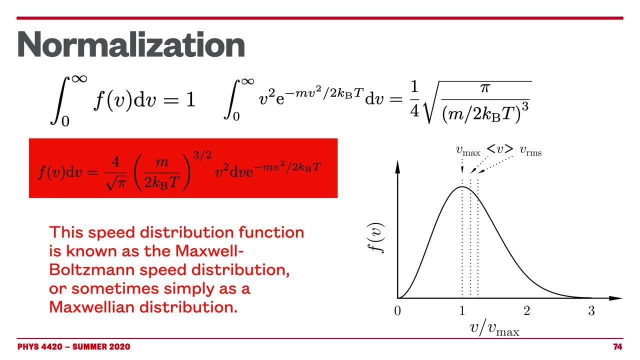 you gives you is the probability of finding the particle, the gas molecule, at a certain uh speed. right, speed is the scalar version, so basically the, the length of the vector. all right, so that's very important because you see that the maximum is no longer at zero um, but it's actually at, at a, as an exponential would be right. the decaying 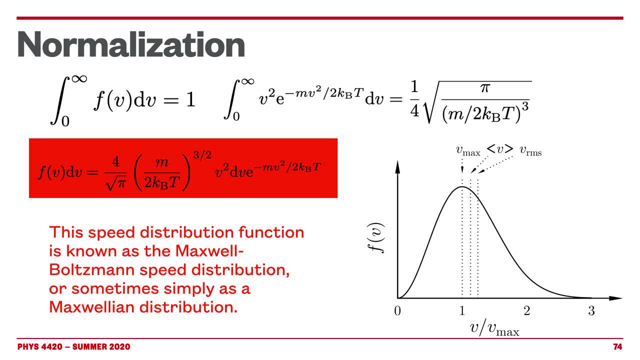 exponential, the maximum is at zero. instead, the maximum is at a finite value, and and the reason why you have this is because you, you have the v square in front of of the equation, okay, so, uh, that's, that's all very good, and uh, we also know that this equation is going to depend on the temperature. i 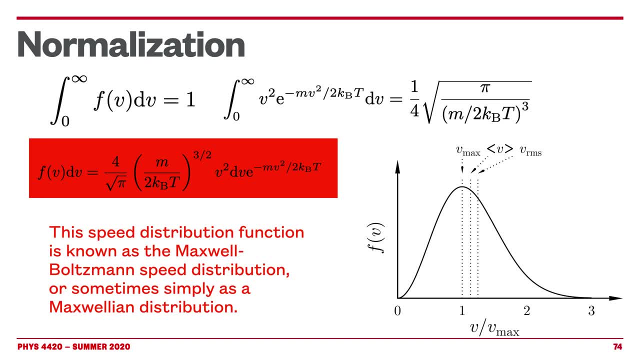 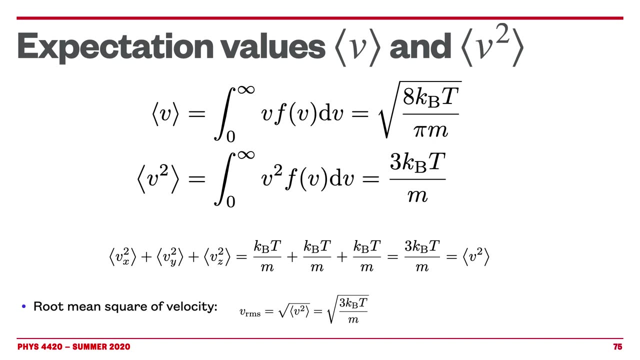 like to attract your attention. there is a temperature in the exponential, but also in the in the pre-factor, uh. one more time, we have a statistical distribution here so we can calculate different things like like the expectation value of the velocity. the expectation value of the velocity is going to be. 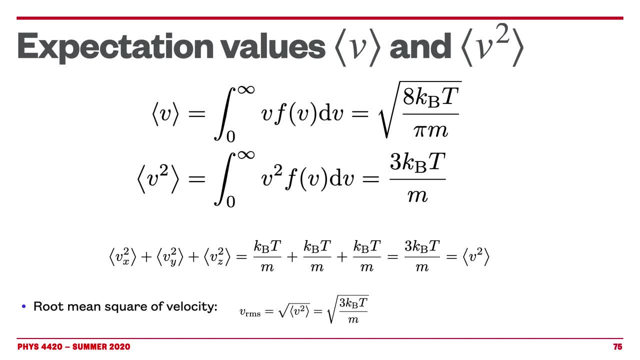 given by another gaussian integral, the expectation value of v square. uh, which is actually very important because the expectation value of v square, as i just mentioned a few minutes ago, is going to be related to the expectation value of the kinetic energy, and what we find is that the 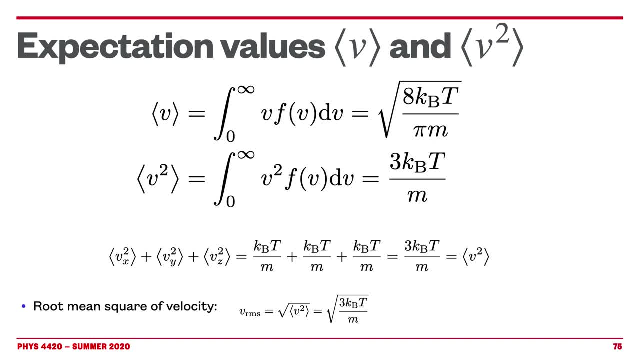 this is a nice bit long, but the expectation value is performisch and is some one kind of like a. basically, what we find is that we have essentially what a kbt over m term contribution for each dimension. so if you had a particle that be confined into one dimension, the 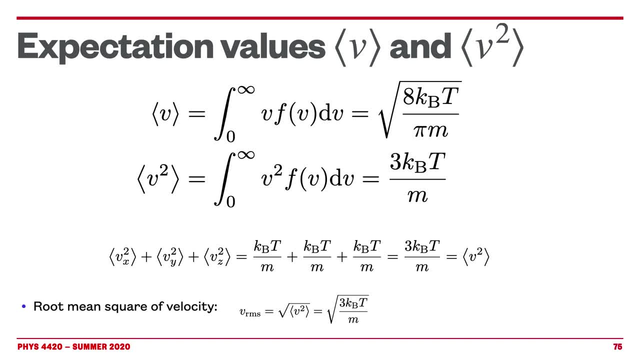 the expectation value of v square would actually be just kbt over m if it were confined in two, And the reason for this is because the expectation value of v square is actually the sum of the expectation value of vx square, vy square, vz square, as we have seen in the first lecture about the expectation value of sums, 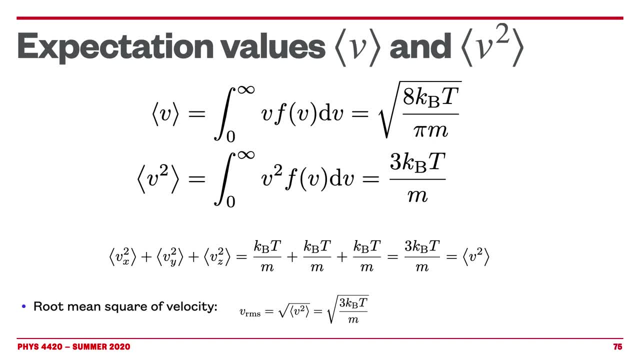 Okay, so we can also calculate the root mean square of velocity, which is, of course, the square root of the expectation value of v square, And that gives me also a statistically important result. So one thing that I already alluded to a few times in this podcast, that I'm going to repeat with the final equation, is the kinetic energy. 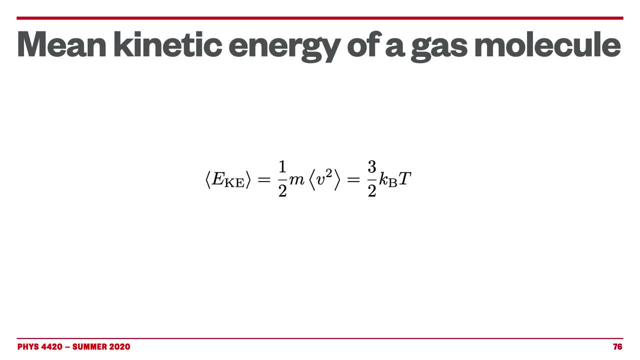 So the mean kinetic energy of a gas molecule in this description we have is going to be equal to 3 half kBT, for the reason I just gave you before. And again, the 3 comes from the dimension. So we've essentially proven a very important result already, right here. 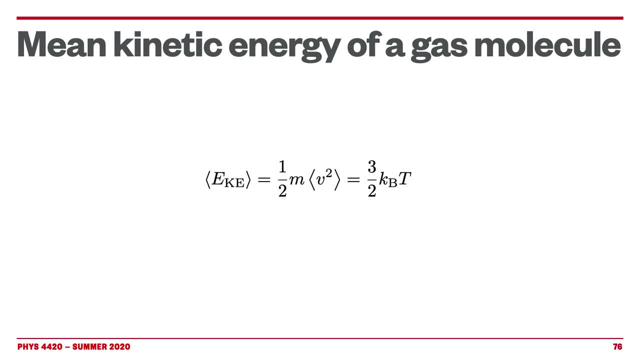 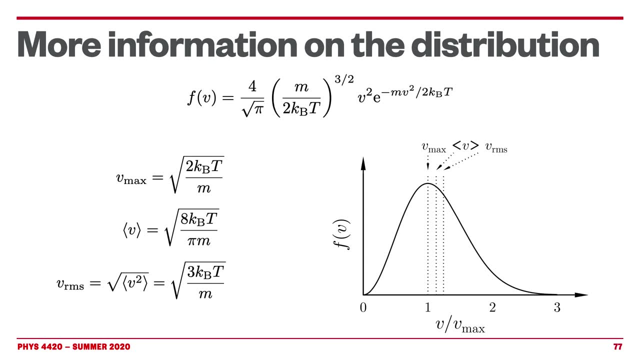 Okay, So just to repeat something that I already said, but in one single slide now, this is essentially a very good summary of what we need to know. The top is the Maxwell-Boltzmann equation, the distribution. We have the value of the maximum. 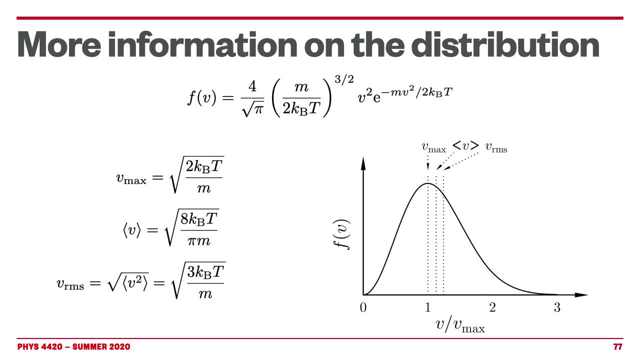 So to find it, you just derive f of v and find the maximum value, the expectation value, and then the root mean square. And when you see this, So you see that they only differ between each other, between a factor of square root 2, square root 8 over pi and square root 3.. 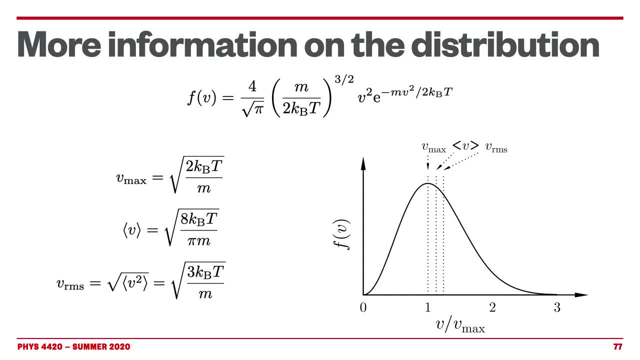 So that means that you see directly that v max is smaller than the expectation value of v, which is itself smaller than the square root of the expectation value of v square. So those three values there can be plotted on the distribution And you see that you have this asymmetric distribution. 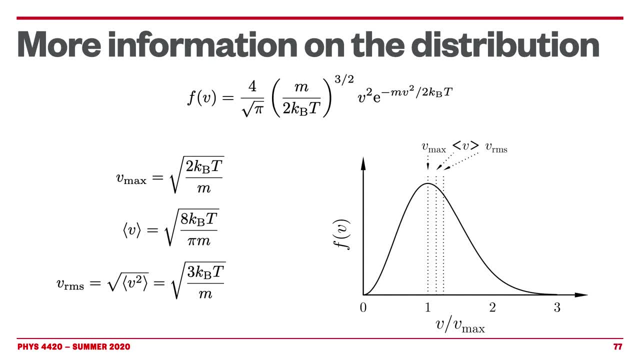 This is the Maxwell-Boltzmann distribution. It's a very good idea to have to kind of have a picture of this distribution in your head And also know what it looks like. I mean, even if you forget what's the pre-factor, it's fine. 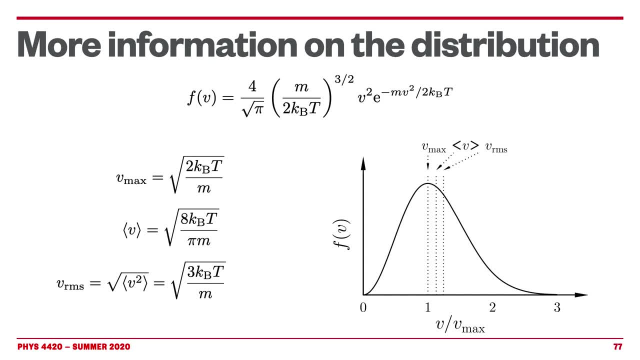 You can find it or can provide it to you. The point is that it's very important to have a picture of what it is. If you go, if you look into the textbook that we are using. there is quite a bit of discussion about how. 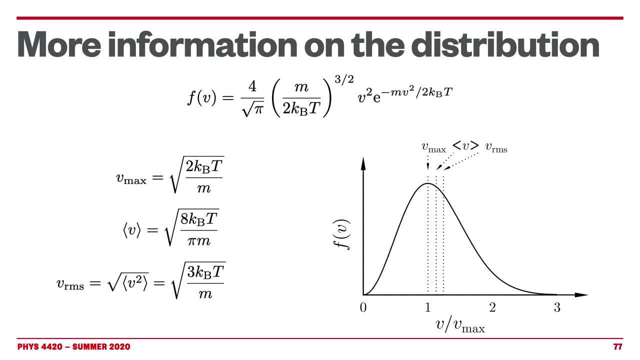 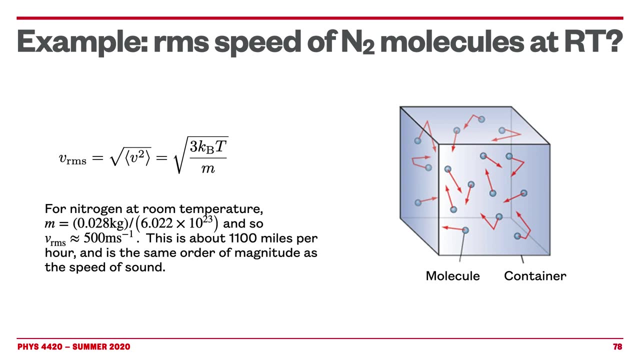 historically, people have been able to measure this distribution and to see that, indeed, it follows exactly this, and it was done successfully. I'm going to skip this part in this, in this, in this screencast, But instead I'm going to show you an example on how to calculate the root mean square speed of nitrogen molecule at room temperature. 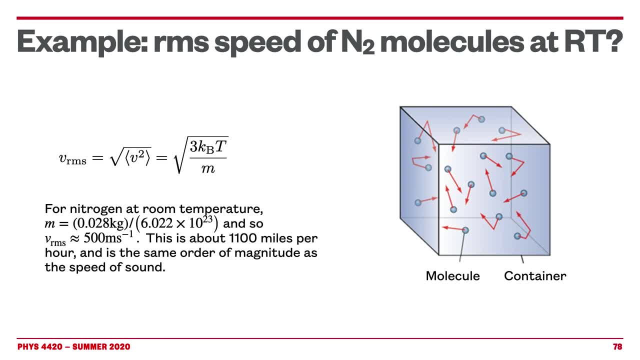 You see that it's actually the only difference that we have. The only thing that we have to worry about in terms of nitrogen molecule is the mass right. So Kb is a constant, T is a parameter of the problem. So the mass, We know the mass. We know the mass of a single of a molecule, right. 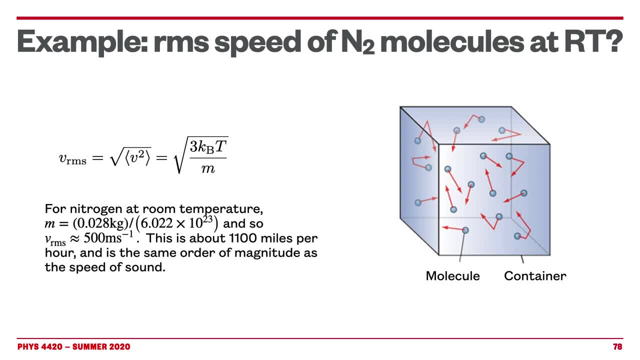 And the mass is just simply given by the molar mass divided by the Avogadro number. and then we find that we find that the velocity, the root mean square velocity of this nitrogen molecule in a gas is about 500 meter per second. Okay, I should say something here. A nitrogen N2 molecule is not. 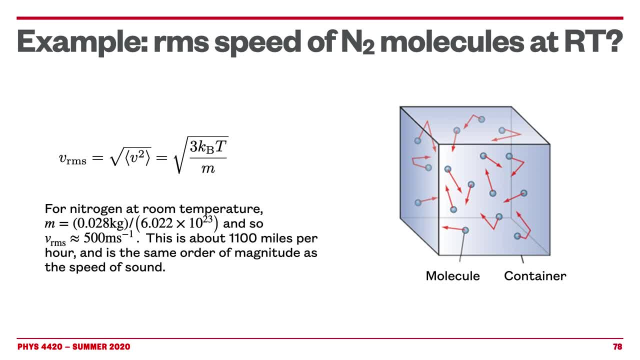 monoatomic or anything like this. But this is so. I understand that what the constraint that we gave ourselves to start with are not exactly met with this molecule. But it's, that's fine, It doesn't make much difference. The point is, the order of magnitude of this velocity is 500 meter per second. I'd like you to realize. 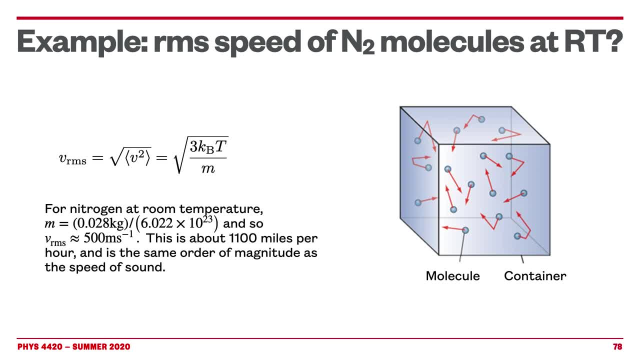 that 500 meter per second is extremely, extremely fast. It's actually about the. it's the same order of magnitude of the speed of sound. So you see this picture we have sometimes of this molecule that I that are moving around and maybe you know, moving. 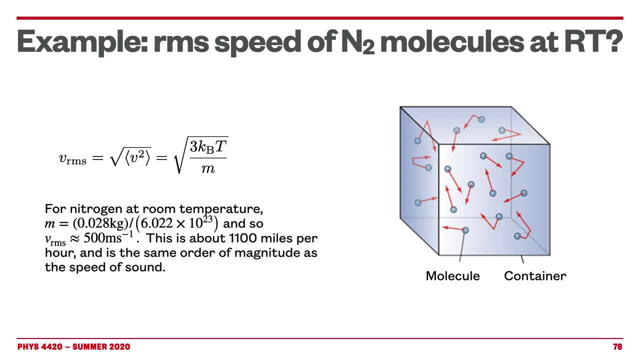 kind of randomly and so on. They do that, yes, but usually the picture we have in mind, the intuition that we have developed over the years from from what we learn, is something that goes pretty slow. We have to realize that when you have a molecule at room temperature, 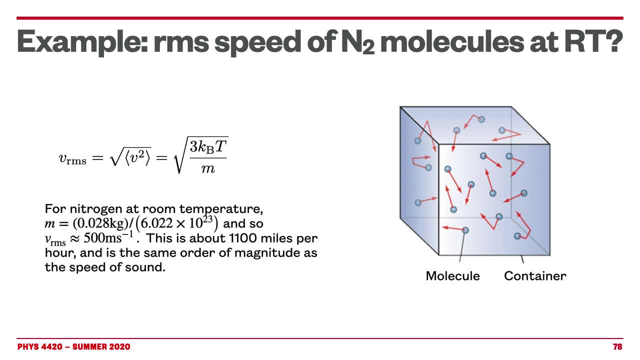 it goes about 500 meter per second. So you have to realize the number of collisions that you have, for example with a vessel or collision with other molecules. They are really the velocity, the pace that's that's relevant to this problem is about 500 meter per second, which is about the speed of sound. 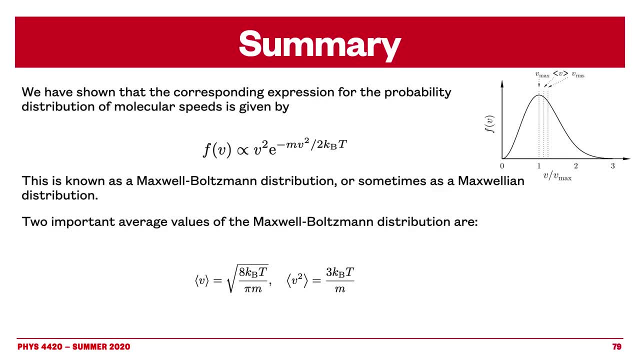 So this concludes this screencast with a summary. The summary is pretty straightforward. We have studied the Boltzmann, the Maxwell-Boltzmann distribution, which provides the probability density of finding a molecule of gas between a certain speed, within a certain speed range, and. 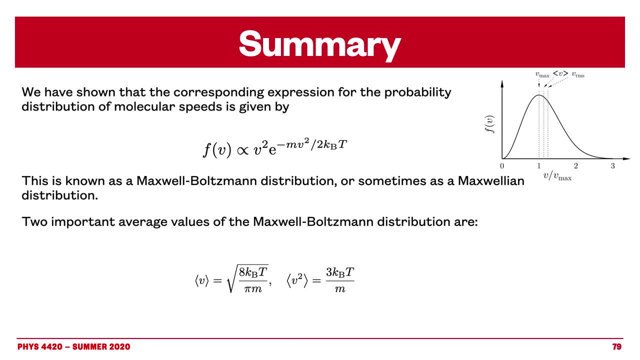 we've studied also the expectation value of V square and expectation value of V. And again, don't be confused Here. the expectation value of V is not zero because we do. no, we no longer have a symmetric distribution, okay. And we don't have a symmetric distribution because we are integrating over all the possible. 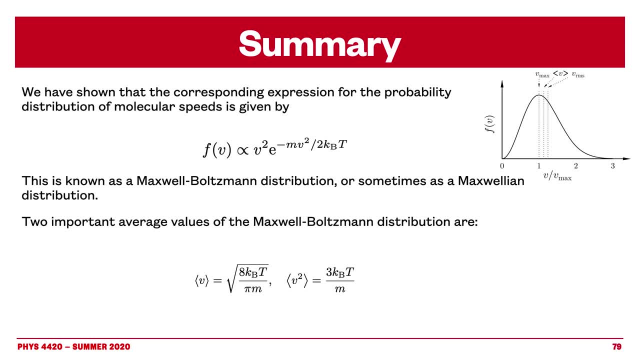 states that correspond to a given speed. okay, Because of course, other different combinations of Vx, Vy and Vz will give us a different value, will give you the same value of the velocity. This is where the, this is where the. 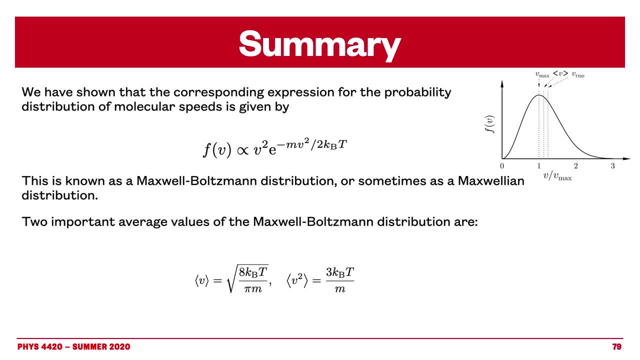 velocity vector actually span. just scan a given shell in a velocity space in Cartesian coordinates. So that concludes our lecture five. The next lecture will be about applying all this to the pressure of the gas. Thank you,